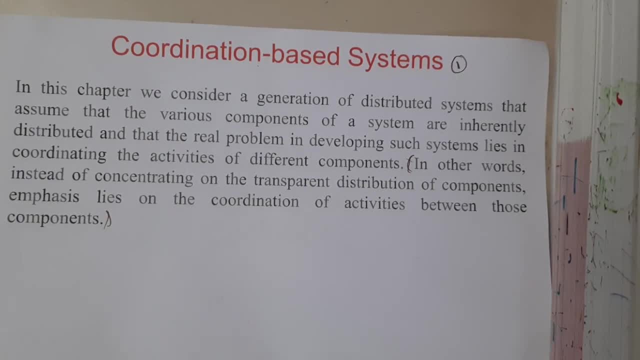 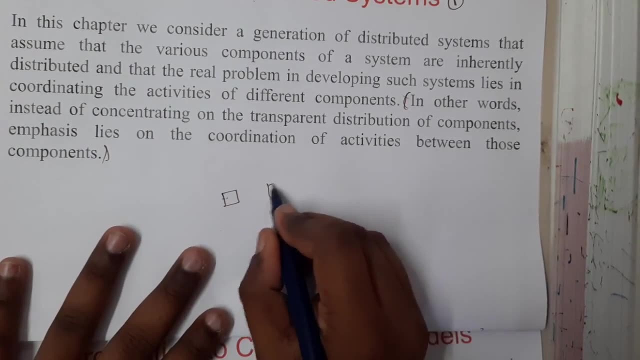 question, right, yes, So once you hear the topic, what is that? what is that? first of all, you need definition, right? yes? okay, So assume till now we discussed about distributed systems, right? yes, Multiple systems are there, they are communicating in between themselves and they are helping. 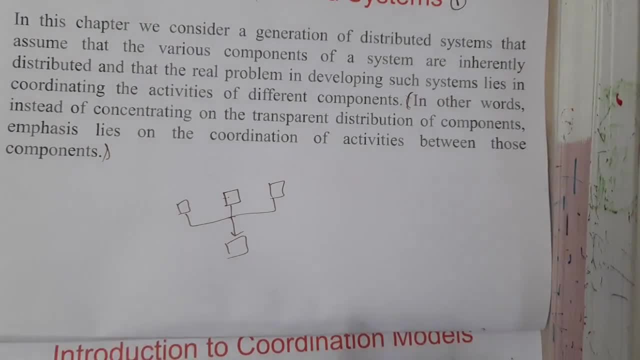 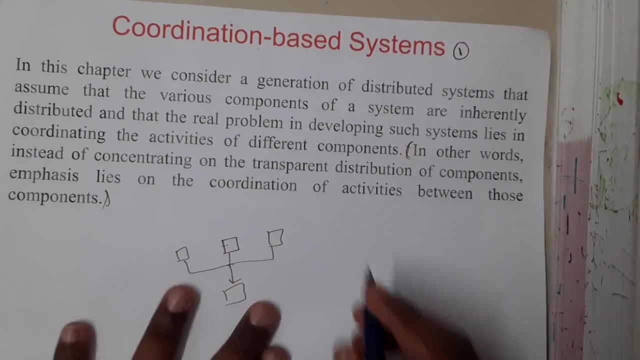 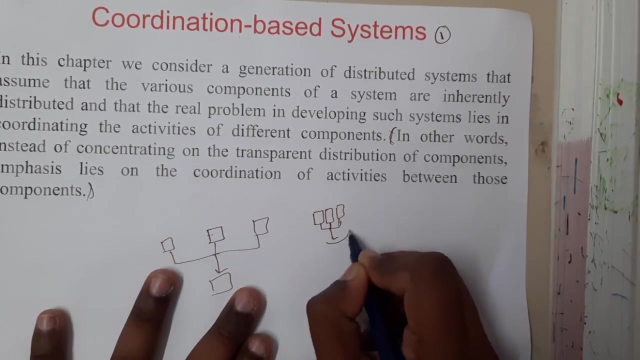 someone to get the data and all those things. So they are distributed multiple places and all those things we discussed, right? yes, Whereas here coordination. so from the name coordination can you understand something, guys? yes, So coordination is nothing but two or more systems will coordinate among themselves to give a result. So this for this sentence: the word 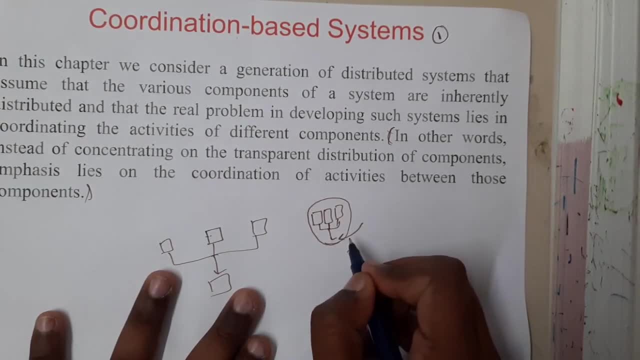 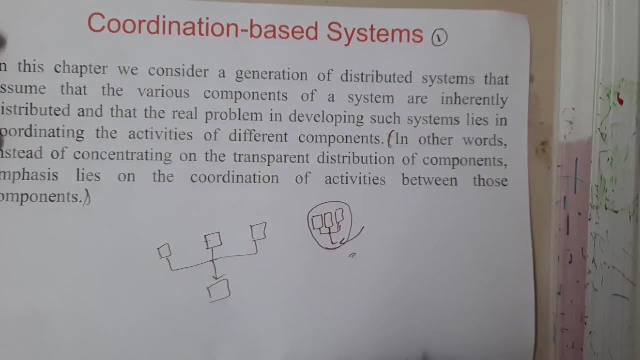 coordination is exactly fitting right. yes, So this process is nothing but coordination, guys. So basically, few systems or a group of systems will combine to do something. Okay, you can go through the introduction part, guys. I'll be going through some some important topic topics or definitions only. okay. So, in other words, instead of 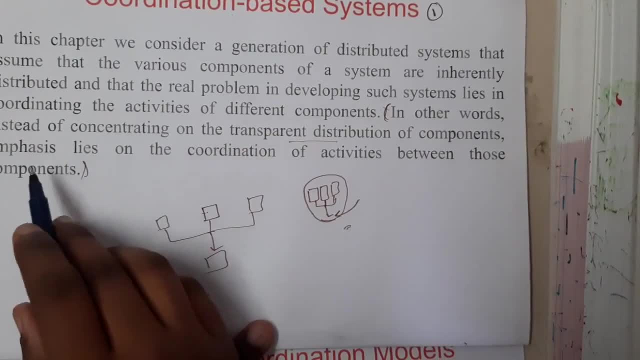 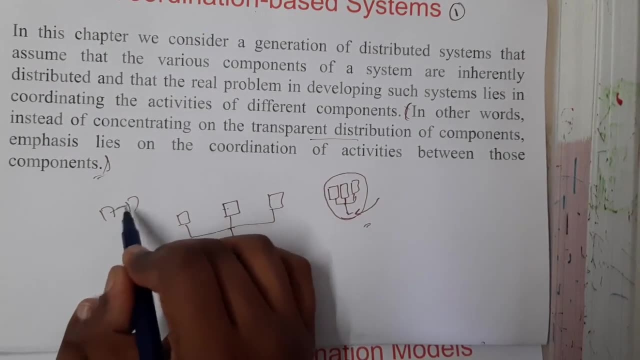 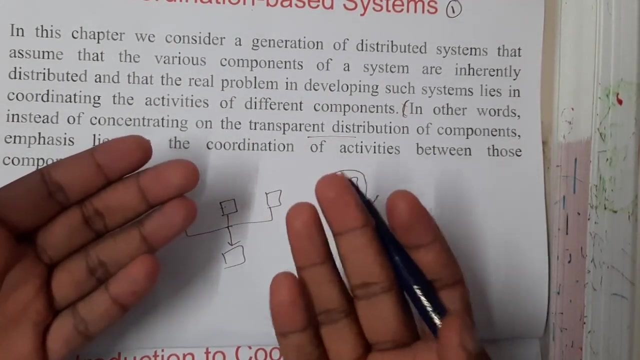 concentrating on the transparent distribution of components. emphasize lies on the coordination of activities between the components. So basically between the components. if you take care of the coordination, how they are, how they are transferring the data, how the this message is helping this message, this component like that, those things, if you check those things. 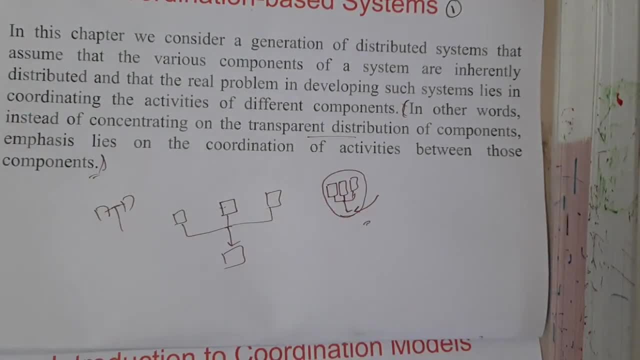 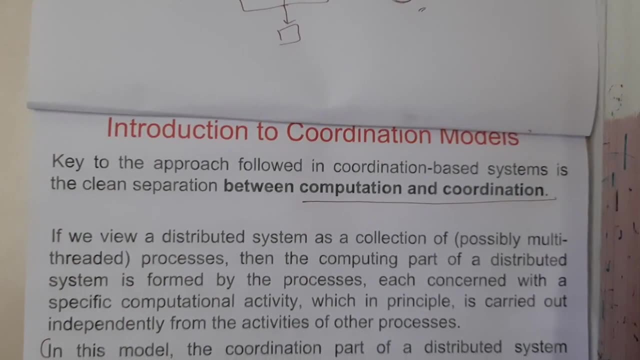 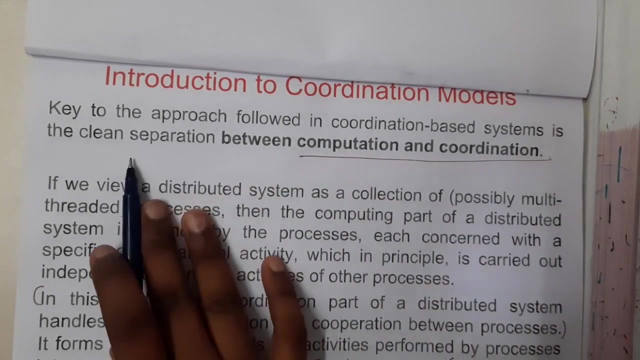 be coming under this coordination based system. guys, okay, so i hope everyone got some basic idea, right? yes, okay, so the key to this approach- okay, just give me a second. guys, okay, so now it's a bit clear, right, okay, so the key to this approach is followed in coordination based system- is to clean. 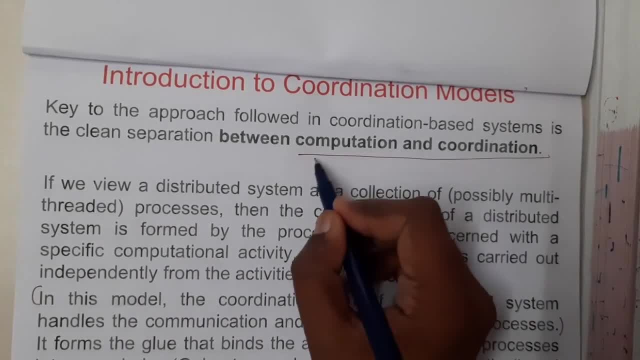 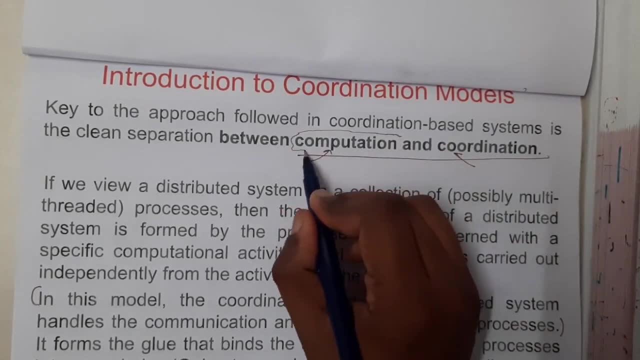 separation between the computation and coordination. so can someone say me the difference between coordination and computation, guys? sorry, computational coordination, so computation. in simple words you can say: it is nothing but calculation, guys. so if i give you x equal to 10 and y equal to 20, and i 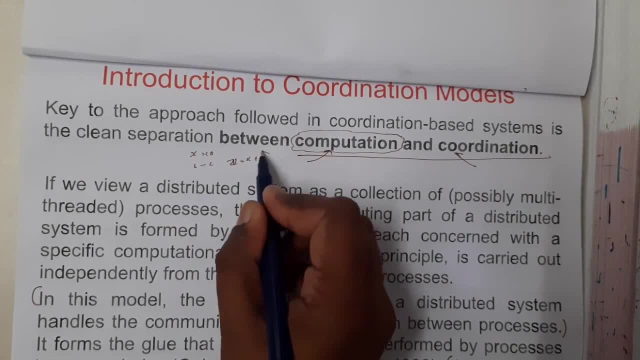 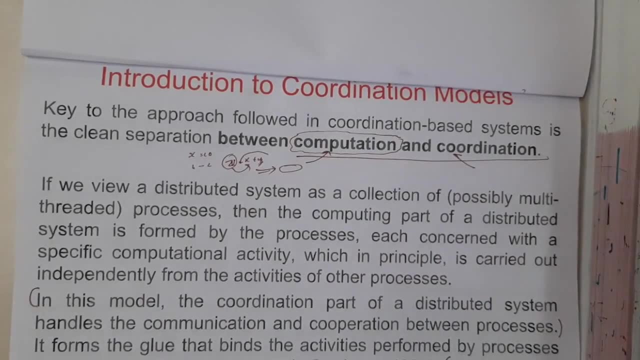 ask you. i ask you: z is equals to x plus y. so i'll be saying: compute the value of z using this. so then you'll be computing it. you'll be calculating and saying with answer: similarly, if i say coordination, so coordination is nothing, but two or few people will be combining and doing something. 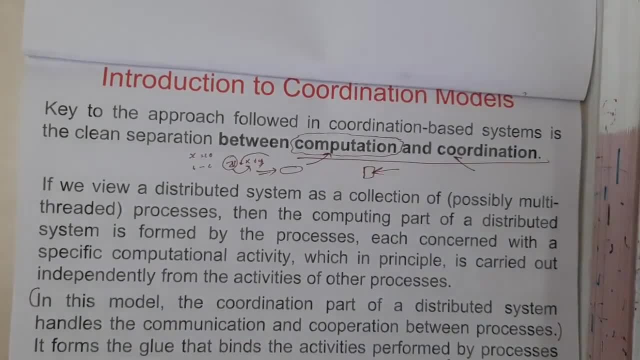 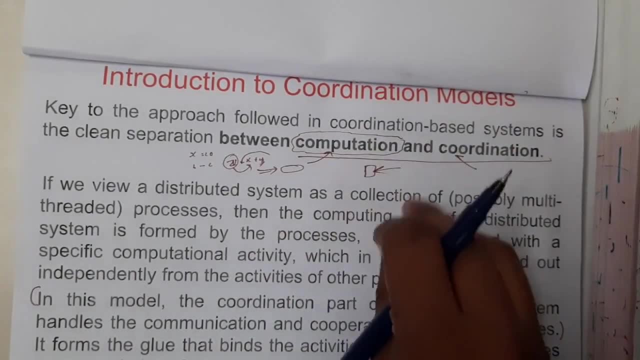 so let us take an example of your major project or your mini project or any kind of project, guys, which you did in a group, right? so you, among your team, you'll be coordinating among yourself and you'll be completing the project. yes, so the same thing will be done. 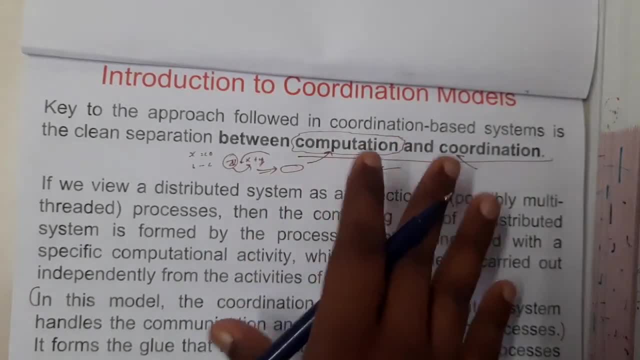 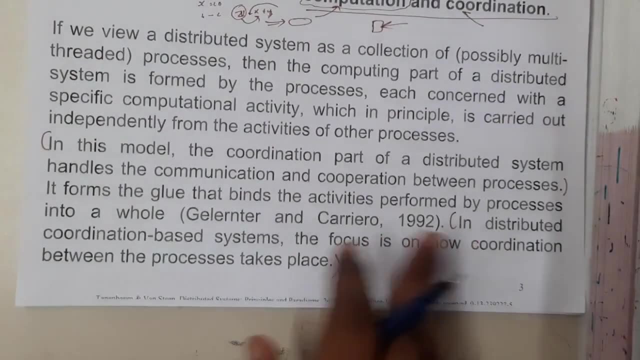 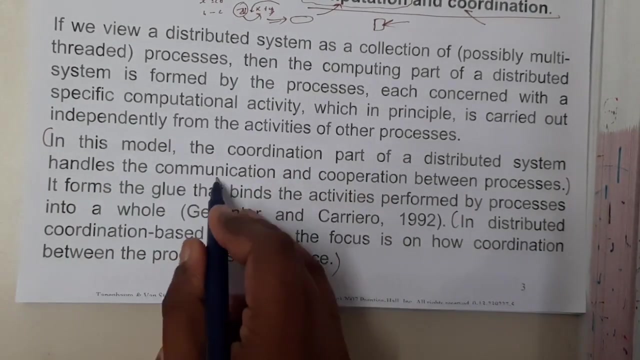 the by the systems or the components here. so that is nothing but your coordination, sorry, coordination based system. so i hope everyone got 100 clear idea right, at least now. yes, okay, so let us continue. so in this model, the coordination, the coordination parts of the distributed system handle the communication and cooperation. so basically they will be: 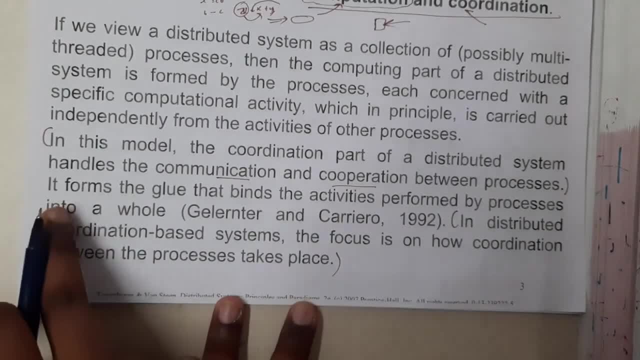 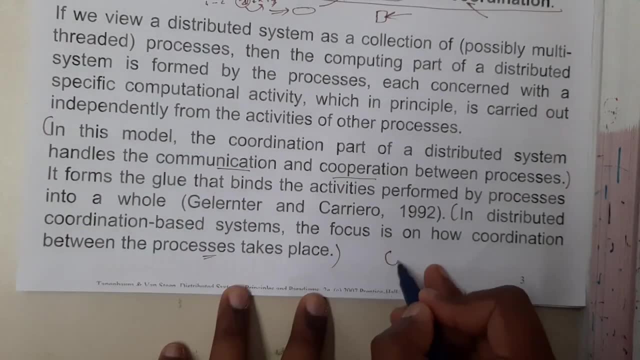 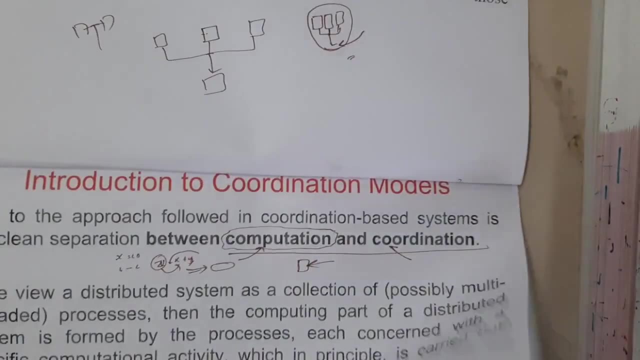 controlling the coordination and even the cooperation, also between the processes. okay, okay. so in distributed coordination system they focus on how coordination between the processes take place, so basically in between the process only, and get the same thing done. so i guess, okay, everyone wants to talk too much. 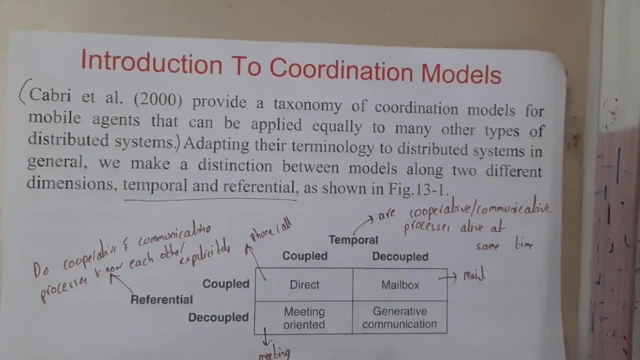 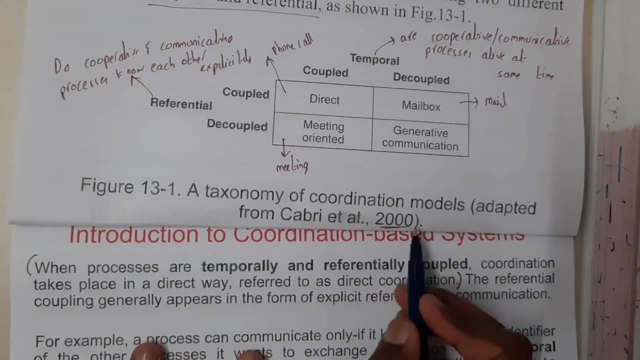 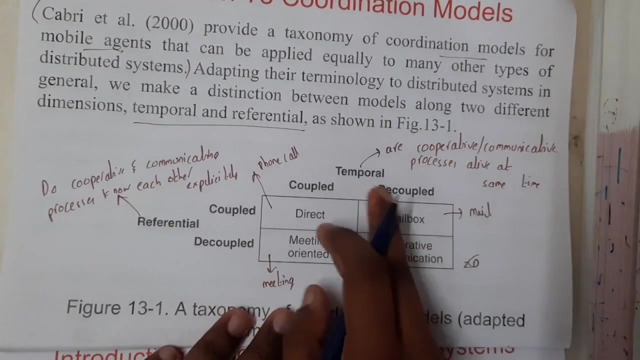 i mean, this can be a form of industries, right, let us know what would be functional and then, just if you are going to moving around with your computer typically, you wanna think of her. and how do we make our decision different? right, and how do we figure out, how can we? your idea of is relatively simple. comp 350 is definitely. 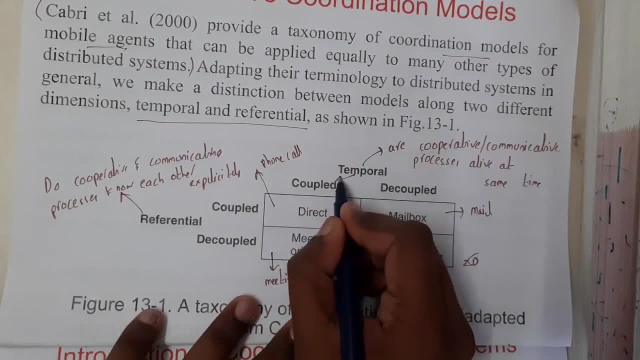 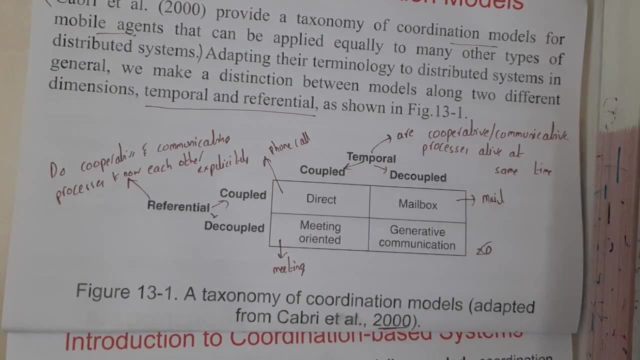 Okay, so on one side, we are having a temporal and coupled and decoupled, Similarly referential coupled and decoupled guys. Okay. so your first question will be: what is this temporal and what is this referential? now? 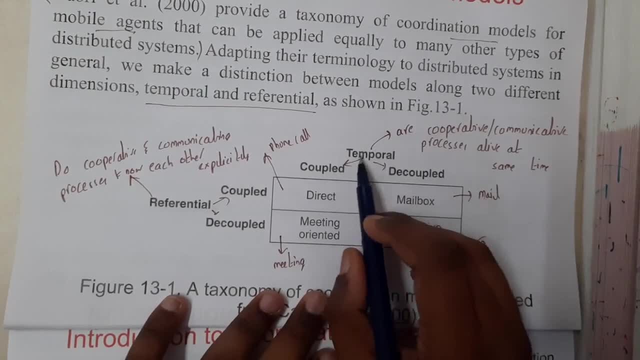 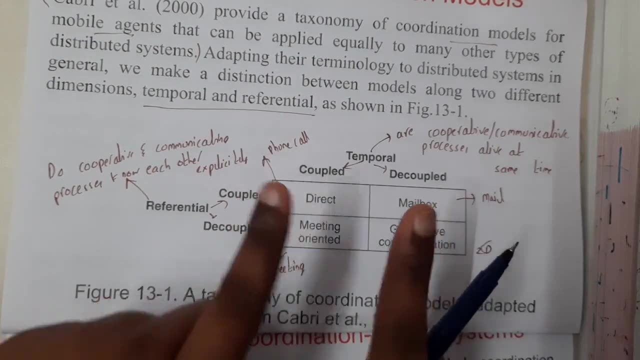 So your question will be that right, Yes, So temporal. So I wrote here itself: Temporal are nothing but are cooperative or communicative processes alive at same time. So basically, if both the processes are alive at the same time or running parallelly, then we can say that they are temporal guys. 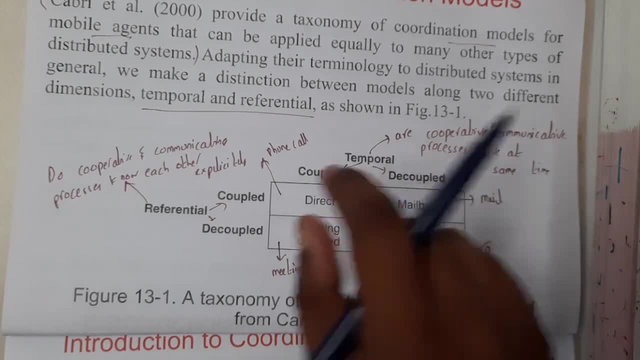 Okay, guys, don't worry about these definitions. Once we are going through the examples, you will be having a clear idea. guys, Don't worry about that. Okay, yes, So temporal means both of them should be alive at the same time. 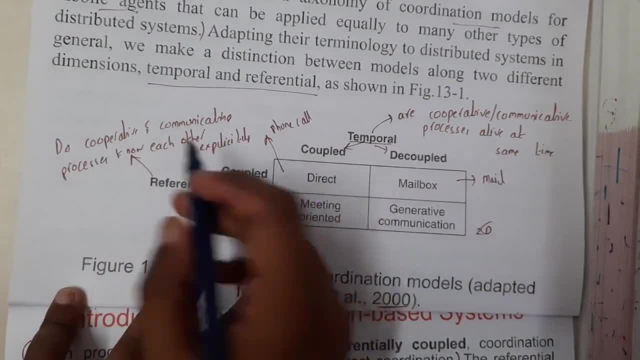 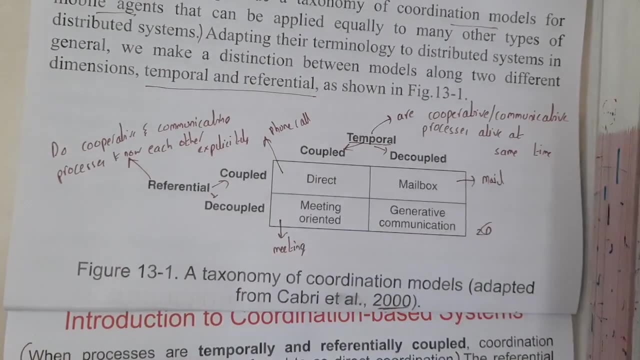 Whereas referential means: do you- this is a question, some kind of question, you can say So do cooperative and communicative processes know each other? So are they known to each other? That is the question there. Okay, yes, 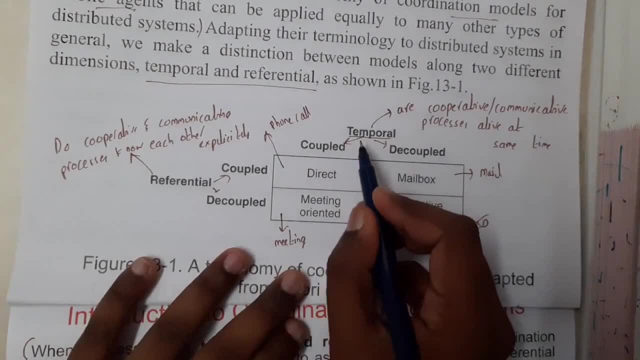 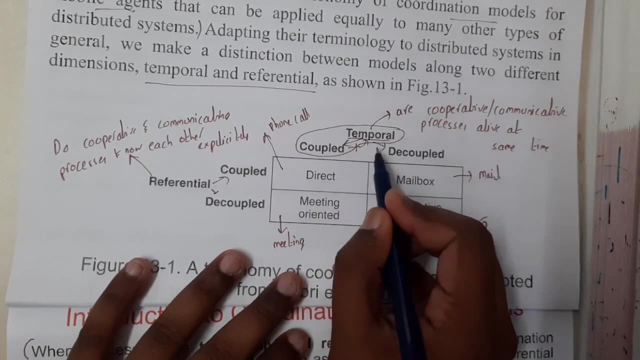 Okay so let us now go through example, guys. Okay, so now observe this word: temporal coupled. So basically, coupled means it is a positive thing, guys, Like this is a true you are saying, Whereas decoupled is nothing but negative thing. where you are saying: this is false. 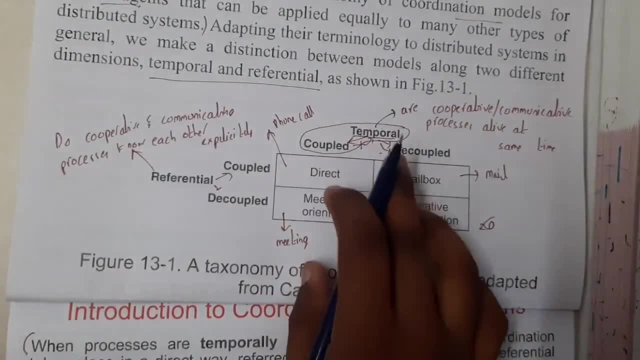 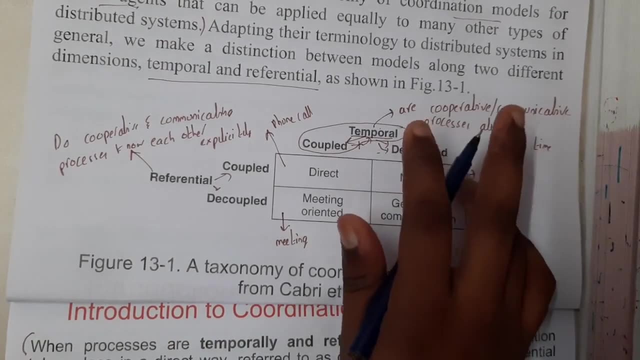 Okay, so while we are going through the example, don't worry, you will be getting. Okay, so temporal coupled means this is a true, I told you right. Yes, So are cooperative and communicative and alive at the same time. 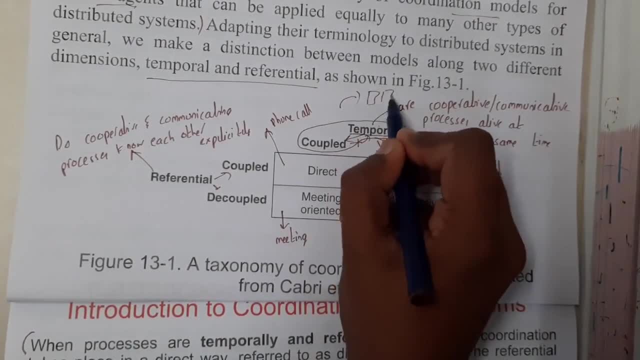 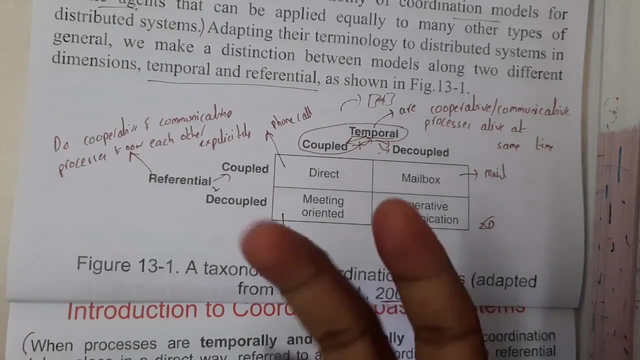 So assume that you called your friend. guys. Okay, and you and your friend are talking. So is it a two-way communication or a one-way communication? guys, It is a two-way communication because you both are communicating at the same time and alive at the same time, right? 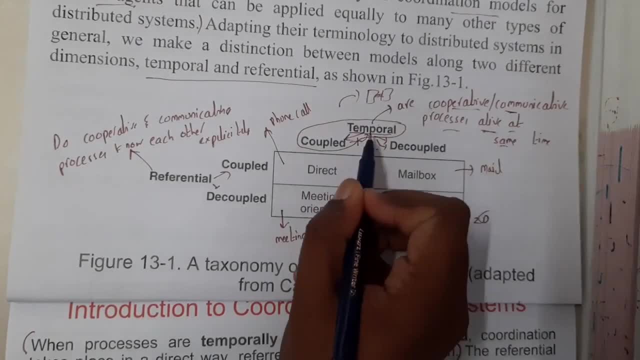 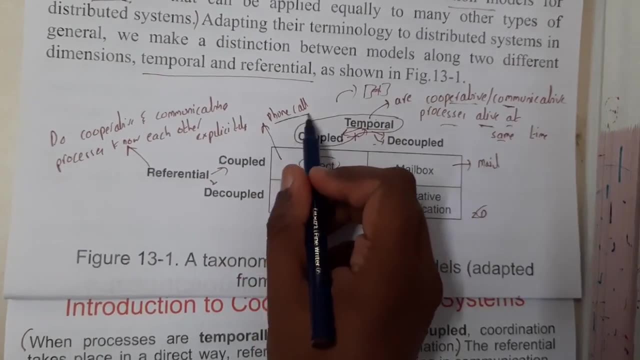 So you are the communication processes alive. So you come under temporally communicated and referentially coupled. So means you will be here, So direct. I gave an example of phone call. Okay. so you might be asking that why I told referentially coupled. 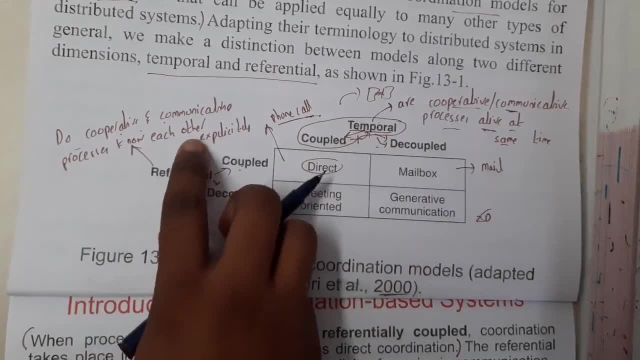 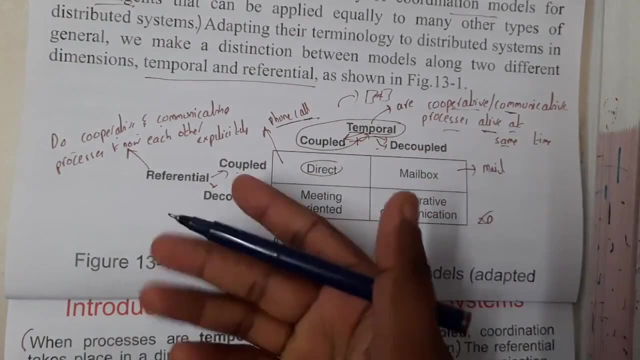 So, referentially, what is that meaning? guys, You both know each other right. So each other explicitly, So you both. you are talking with your friend because you know him right. If he is an unknown number, you will be just talking for some time and you will be disconnecting the call. 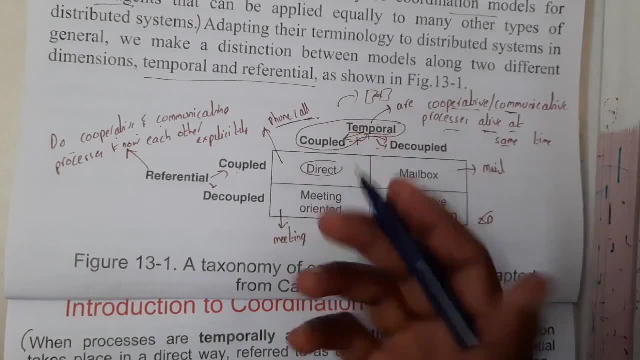 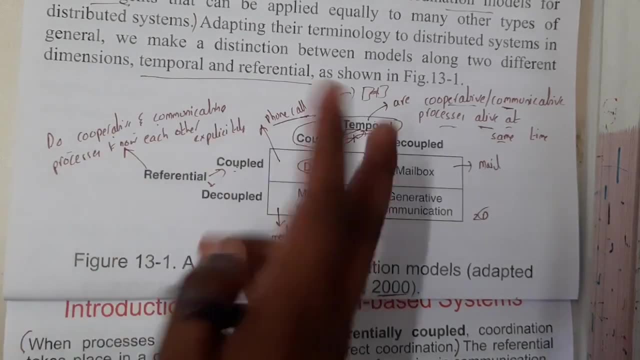 But you are talking for a long time means you are known friends and you are temporal Means you both are communicating at the same time. Yes, That comes under here. Similarly, you know both of you, You know, you know both. sorry. you know your friend and you are not alive or you are not talking at the same time. 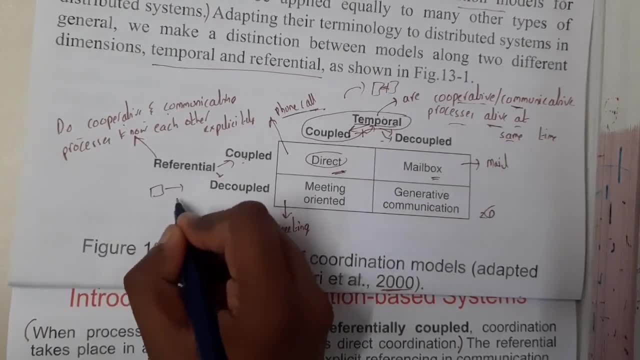 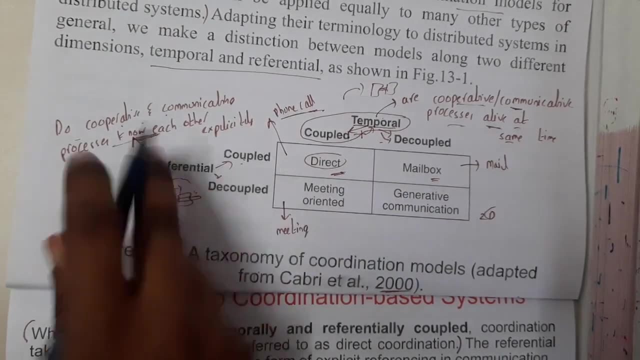 So that could be a mailbox, right? So you might be sending a mail to a person. You should know that person's email address before you send, So you are indirectly having an idea who is that person. So that is the reason why it comes under referentially coupled and temporally decoupled, because you both are not talking at the same time. 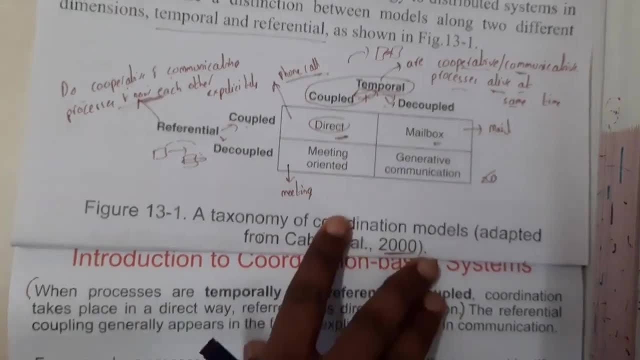 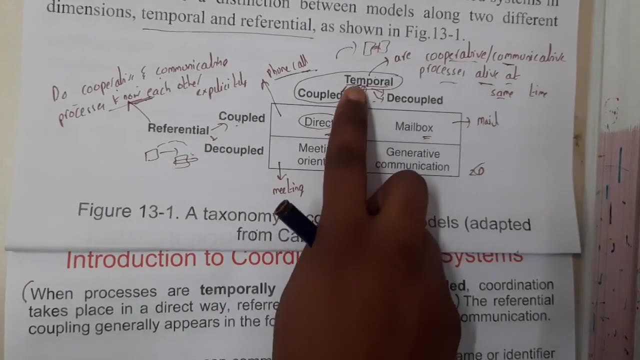 So you both are not sending mails at the same time, right? Yes, Okay, So now let us continue. Referentially decoupled means you are unknown to each other. Referentially decoupled and temporarily coupled So means you both are alive at the same time. 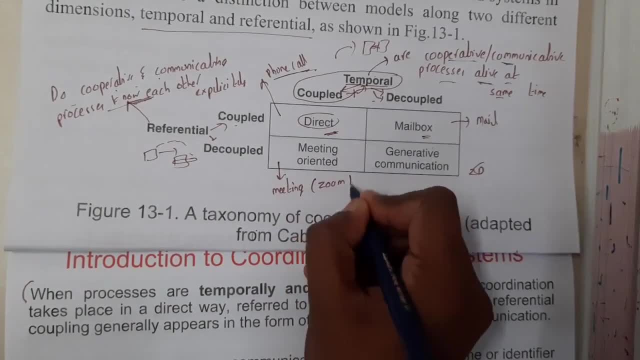 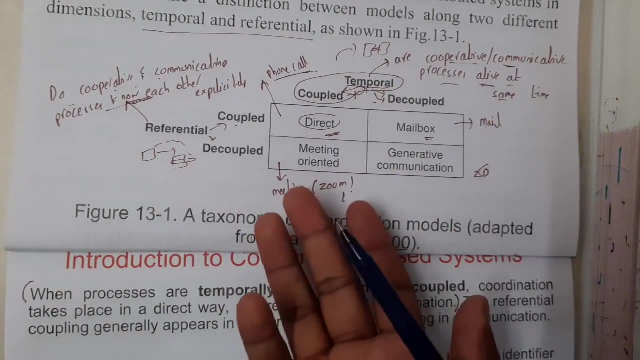 So the best example for this will be your Zoom meetings, guys, Zoom meetings. So basically assume that you got a mail, that there is some special class of unknown. You got a mail from unknown member, unknown email ID or some particular company. 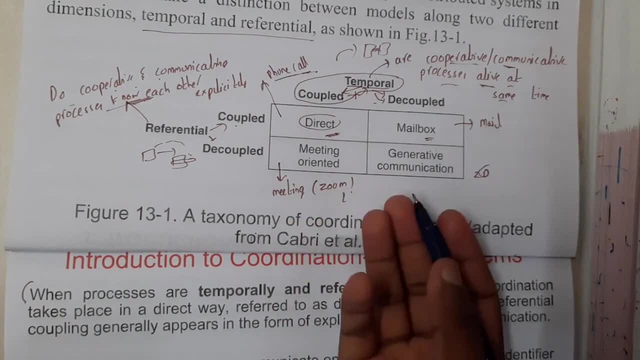 Yes, Let us assume So there is a guy who is teaching some kind of programming language, So you just joined. So in that situation you don't know who he is, But you can. You can communicate with him, right. 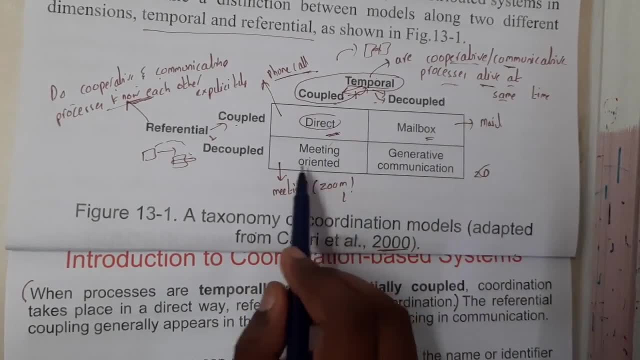 Yes, So you both are alive and you can communicate with him. So that is the reason why it came here. Similarly, referentially decoupled means you don't know both of you. You don't know each other, Okay. 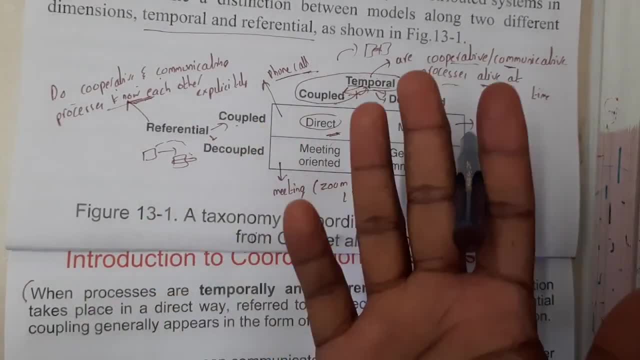 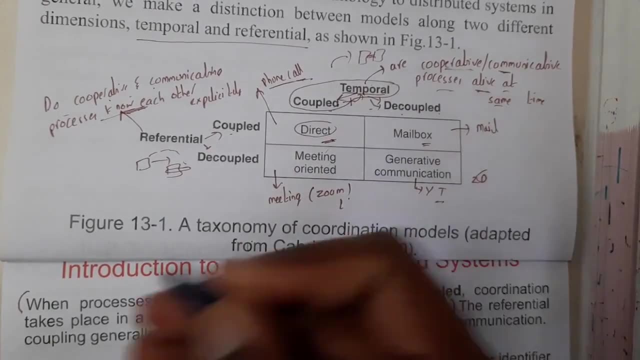 Similarly temporarily discoupled. That is nothing, but you don't know who he is. also, Right, I mean, you both are not alive, So for this, the best example could be your YouTube videos, guys. Okay, So you don't know whom you are listening to. 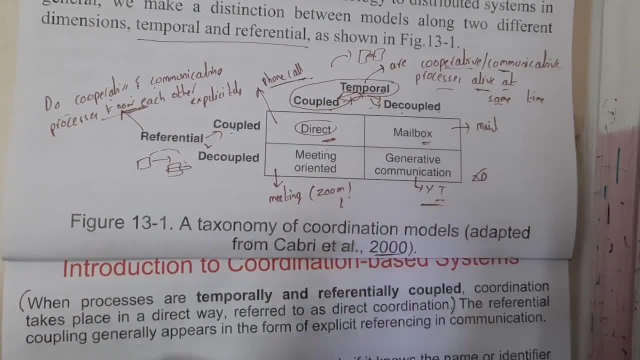 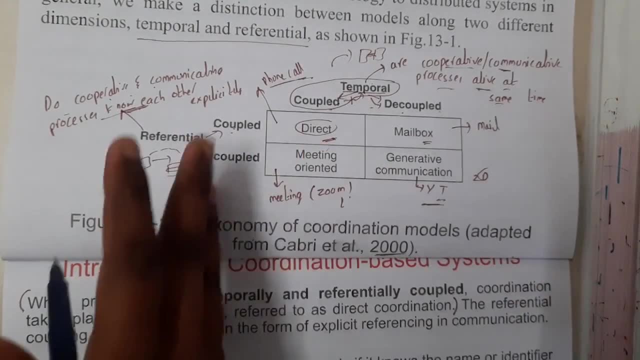 Okay. So I am not saying in all the cases, but in most of the cases Okay. To whom you are listening? you don't know, And And both of you are not alive at the same time. I mean by alive is nothing, but you are not communicating with him in life. 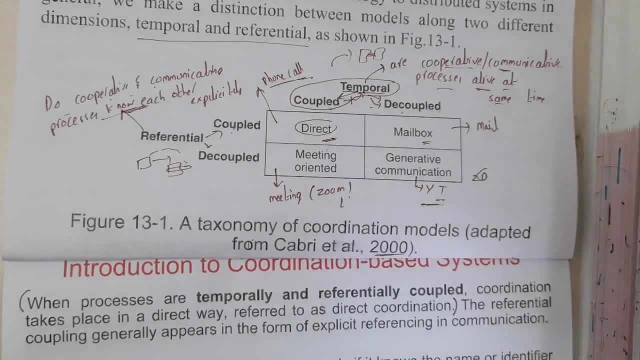 Right, Yes, So now I hope everyone got some basic idea about this box, Right? Yes, I gave some real-time examples, guys, So that you can remember it really easily and clearly. Okay, Yes, So let us continue. 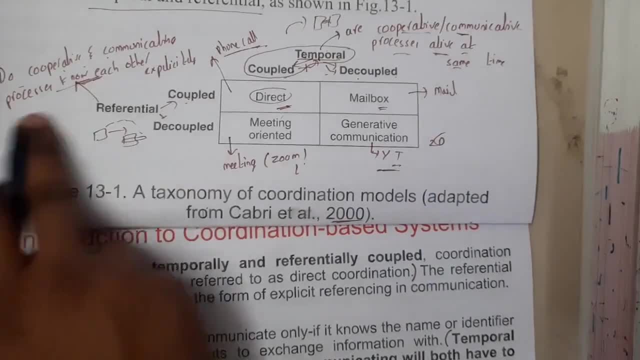 Okay, So those are the exact statements, guys, If you, I wrote here Right. So these statements are already written in the theory part. But in the theory part, if I start reading and searching, that could be an issue. 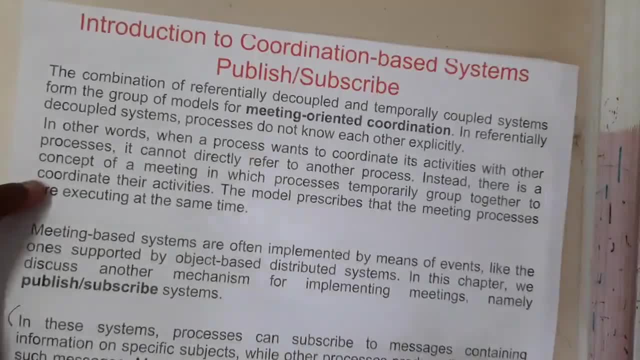 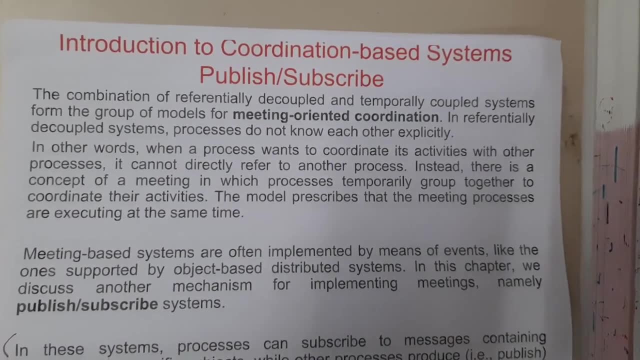 So that is the reason why I have written them aside, guys, Okay, Yes, Okay, So you might. You might be having it Okay. So now we got some idea about this coordination-based system. So are there any real-time examples for this type of systems? 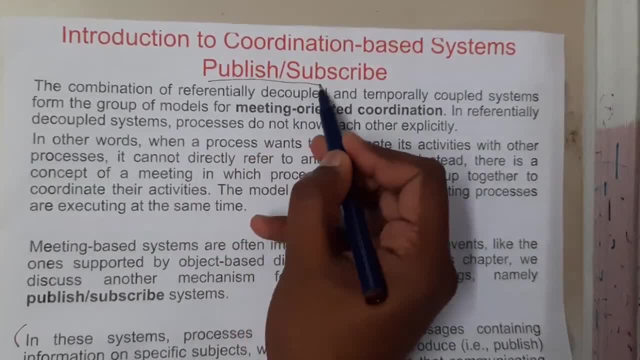 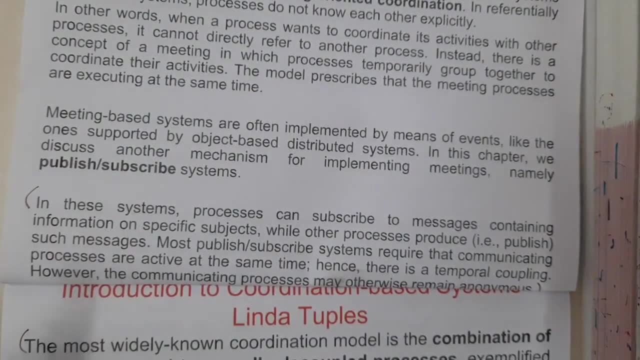 Yes, There is a one popular system, guys, That is nothing but publish and subscribe system, guys. I think the names itself clearly says to you guys, It is just like YouTube: You can subscribe and whatever we publish, you can watch. 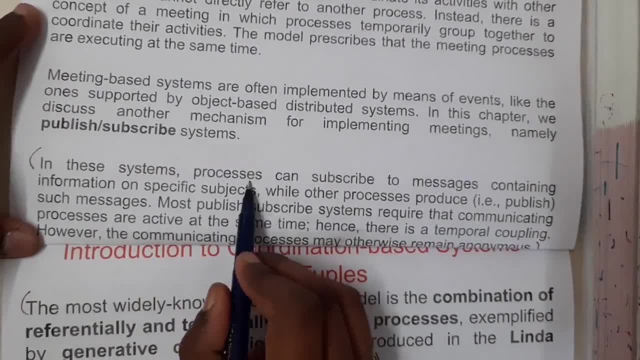 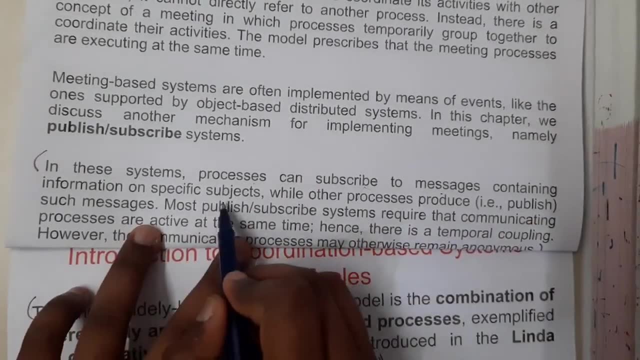 It is the same concept here also. Okay, So in these systems, processes can subscribe. So basically, assume that you are the processes and you can subscribe to the messages Containing information on a specific subject. So, based on the subject and based on your requirements, you will be subscribing to us. 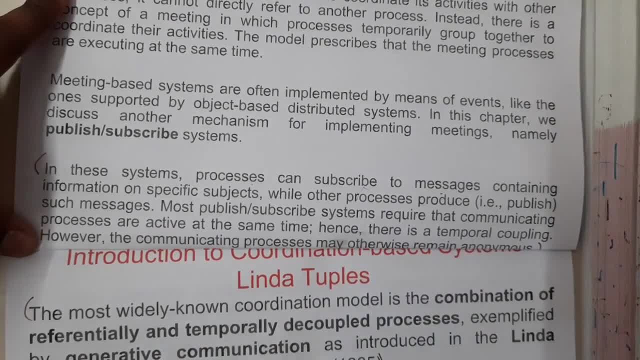 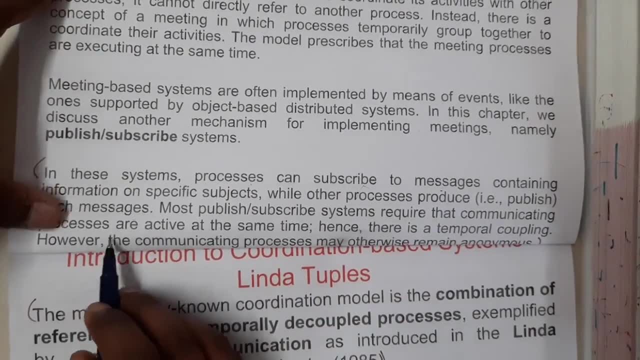 Okay, So, while other processes, that is, publisher, So we will be publishing messages, So we will be sending some messages. Okay, So most publishers and subscriber systems require that communication process are achieved at the same time. So basically both will be do. 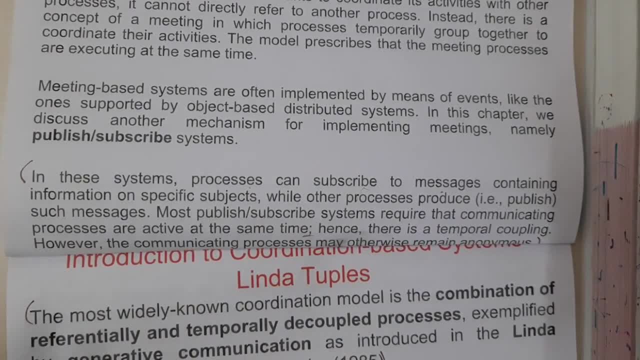 We can do at the same time. Right, You can watch my other video and I can also upload at the same time, Right? Yes, So in the same way. So hence this is a temporary coupling. Okay, So temporal coupling. 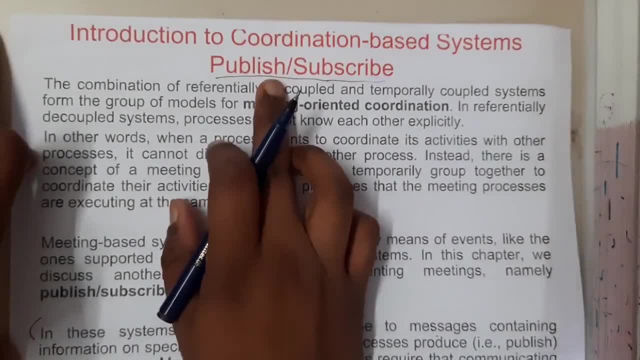 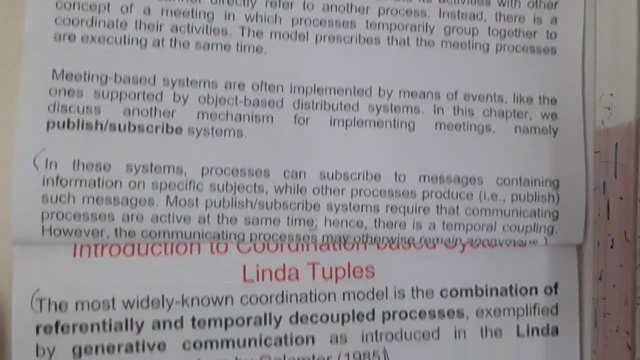 Okay. So now? Now I hope everyone got some basic idea of real-time example of a publisher publish system. Right, Publish, Sorry, Publish and subscribe system. Publish or subscribe system, Okay, Okay. Similarly, we are having one more system, guys. 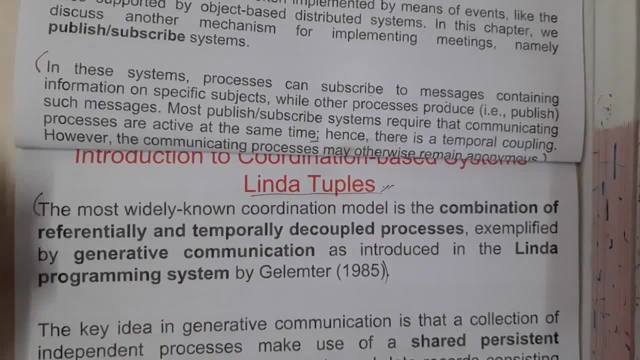 That is nothing but Linda Tupple. So, but I did not got that much clarity, guys. So just to go through it on your own, guys, Because I don't want to confuse you with some kind of wrong things. That's the reason why I am just skipping it.